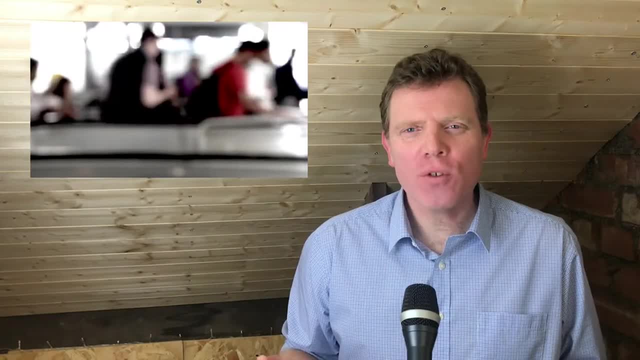 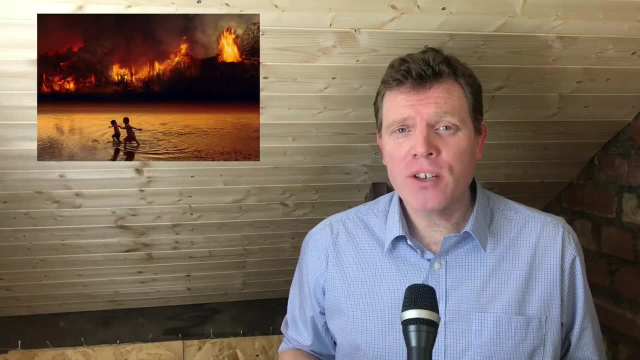 It's really important that we, as humans, recognise that our actions have consequences. We're burning vast quantities of fossil fuels that are releasing enormous amounts of greenhouse gases. Along with deforestation and other industrial processes, these will all lead to an enhanced greenhouse effect. 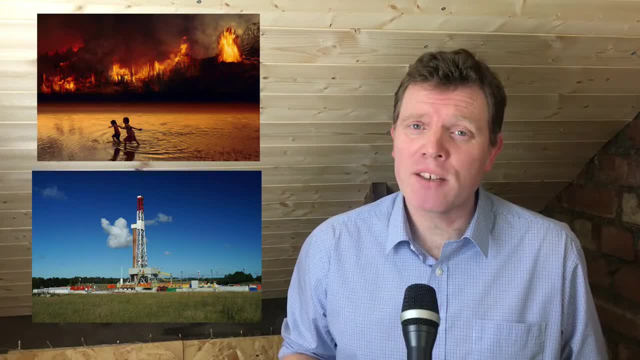 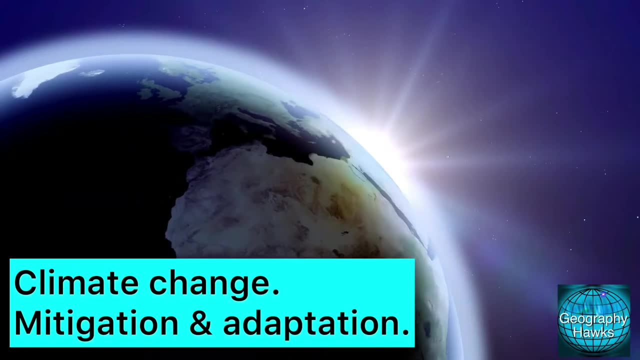 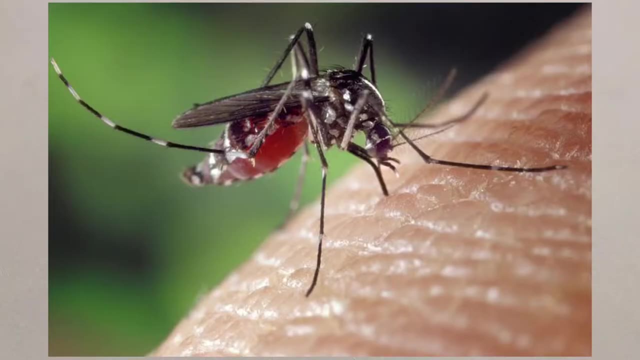 What we have to do is find ways to mitigate the threat that we face. There are numerous impacts of global climate change: From stronger and more frequent tropical storms to heat-related diseases like malaria, From increased drought and flooding to desertification and loss of habitats. 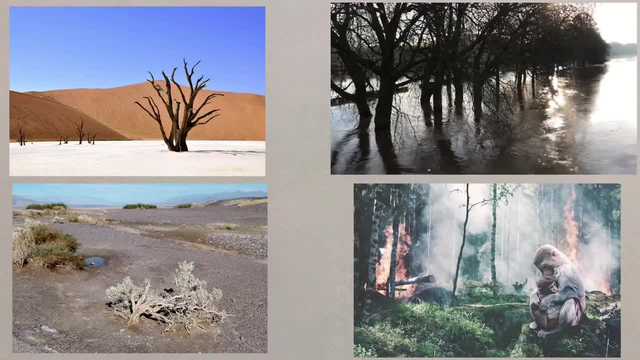 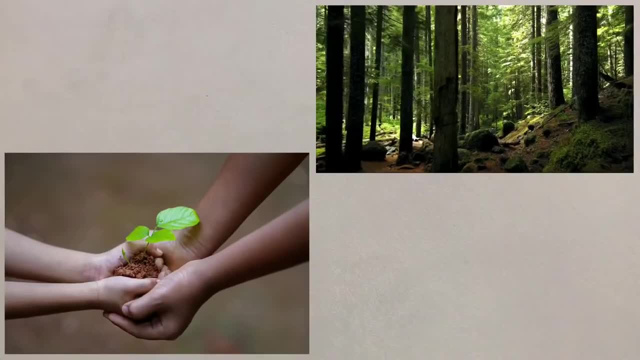 With so many potential impacts from global climate change, steps need to be taken straight away to mitigate these impacts. A simple method of mitigation is to plant trees. Trees absorb carbon dioxide for use in photosynthesis and can release moisture into the atmosphere through transpiration. 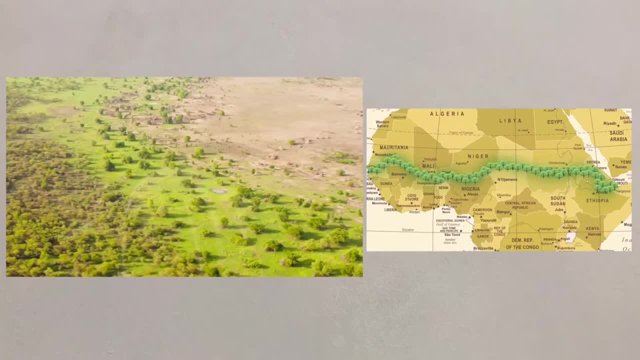 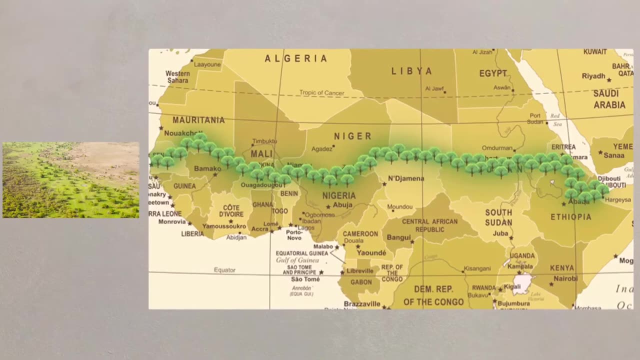 This moisture will help to cool the atmosphere. One such programme is the Great Green Wall in Africa, set to create an 8,000-kilometre wall of trees stretching right across the continent. Alternate renewable energy sources can also help mitigate climate change. 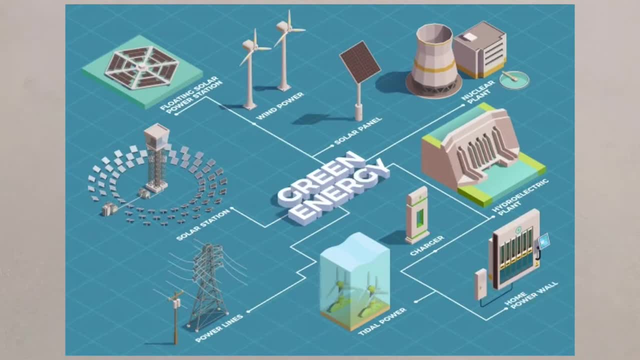 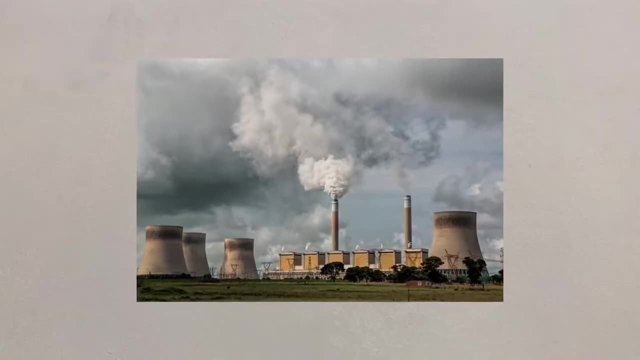 Hydroelectric, solar, wind and tidal, to name a few, are all sustainable, renewable and don't emit greenhouse gases as a by-product of their energy generation. Carbon capture and storage uses technology to capture up to 90% of the carbon dioxide emitted. 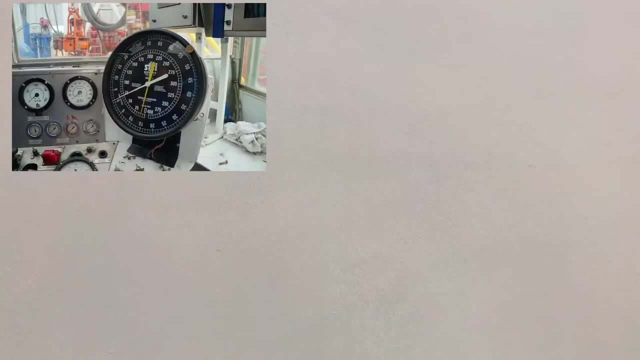 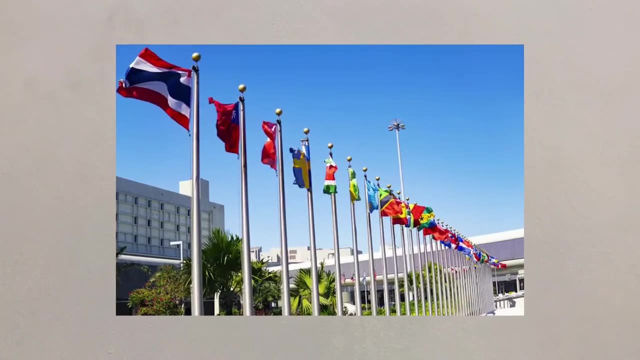 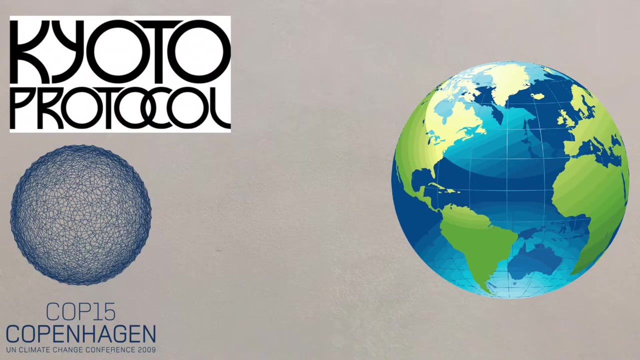 when fossil fuels are burnt. When it's captured, it's then compressed and transported through pipes to a well where it's injected as a liquid into the ground. International agreements are important because the climate affects the whole planet: The Kyoto Protocol of 2005,, the Copenhagen Accord in 2009 and the Paris Agreement in 2015. 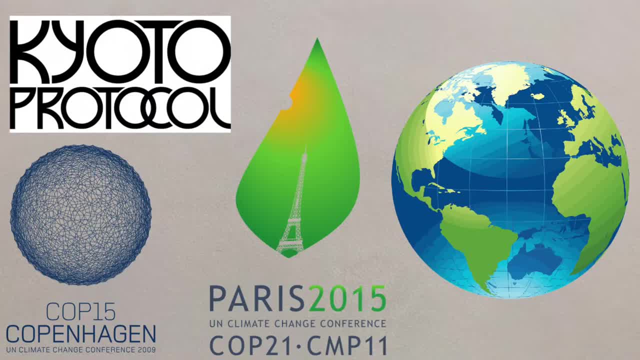 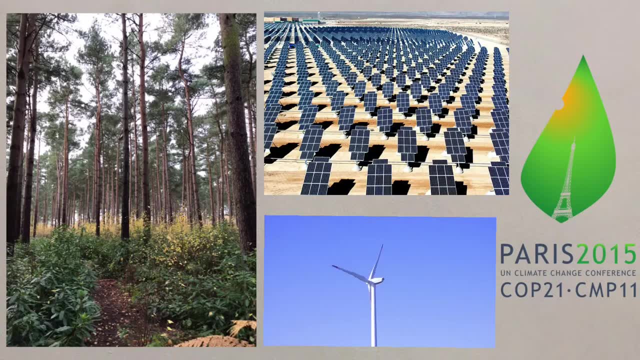 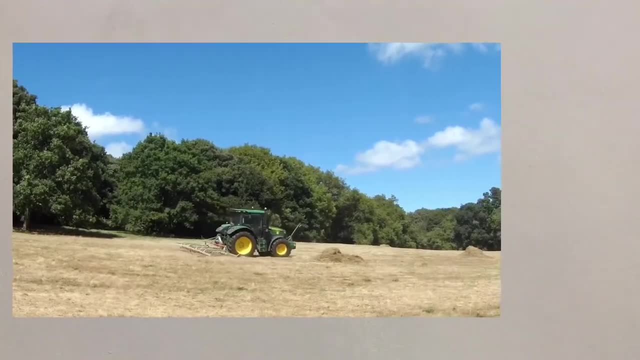 have all aimed to tackle climate change and reduce the emissions of greenhouse gases. Mitigation is crucial to reduce the effects of climate change, But we also need to adapt to the changes that are here and those that may come in the future. Agriculture will need to adapt because, although scientists believe that in middle latitudes, crop yields from certain crops will increase,